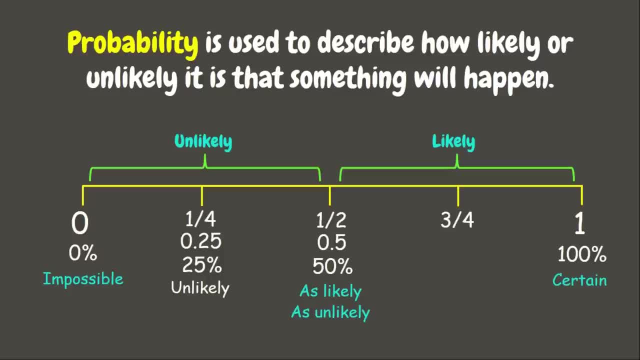 For example, if the probability is 3 fourths, which is 0.75 or 75%, the likelihood of the event to happen is likely, since it's between 1 half and 1, or 50% and 100%. Now let's go back to our problem. 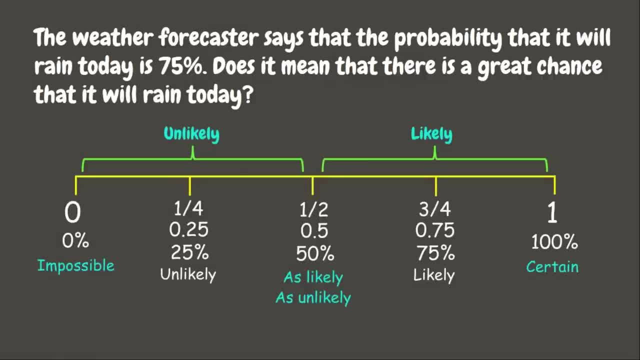 Let's use our probability line to determine the chance that it will rain today. Since the forecaster says 75%, we can see that 75% falls between 50% and 100%. This means that the event that it will rain today is likely to happen. 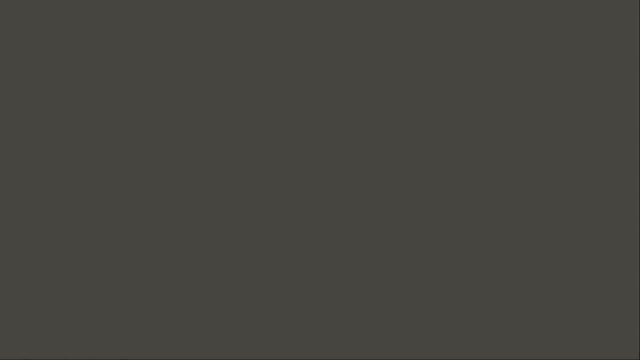 Great job. Now let's determine the likelihood or probability of the following events using our probability line. First is it will snow tomorrow in the Philippines. We all know that the probability of the event to happen is 50%. We all know that the probability of the event to happen is 50%. 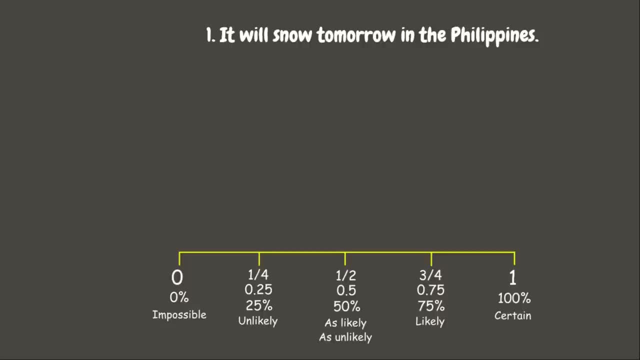 We all know that there's only two seasons in the Philippines, which are dry and rainy seasons. It means that there's zero probability, or it is impossible to snow in the Philippines. Second one: the sun will rise tomorrow. Since sun rises every day in the morning, it means that there's 100% probability, or it is certain that the sun will rise tomorrow. 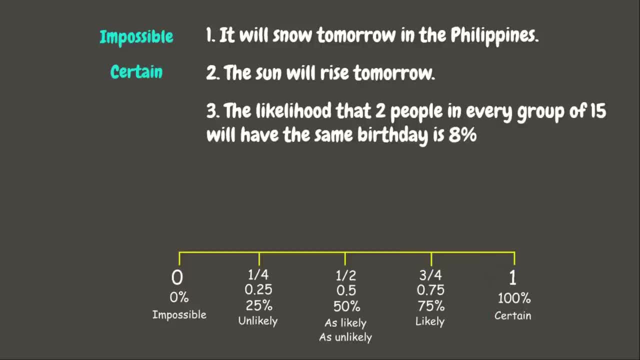 Next one, the likelihood that two people in every group will be able to snow tomorrow. Since the probability of the event is 0,. it means that all the groups in the group of 15 will have the same birthday, which is 8%. 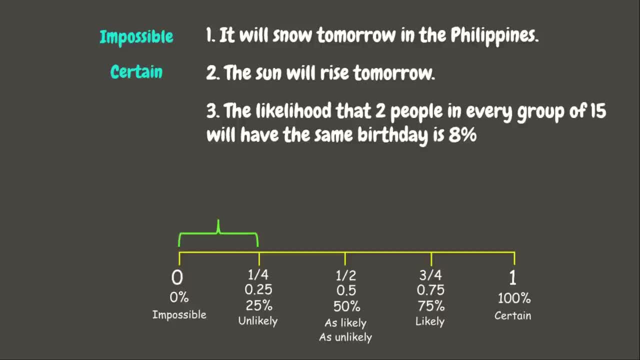 Since 8% is close to 0, and it falls between 0% and 25%. therefore, the event is unlikely to happen. Next, one Sport Analyst says that Manly Pacquiao has a 85% winning, Since 85% is close to 100%. 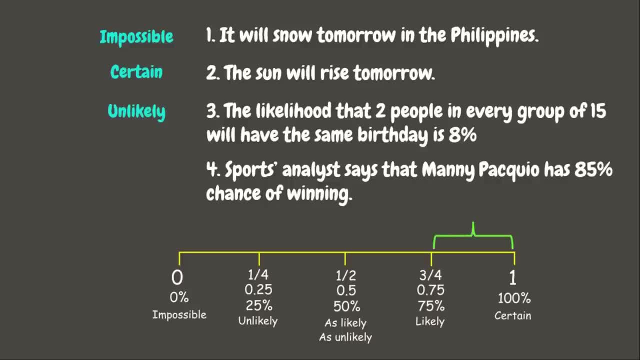 which falls between 0% and 75%. it means that the event is likely to happen. It means that the event has 80% chance of winning likely to happen. wonderful, now let's have another example. let's say in a box there's one yellow cube. 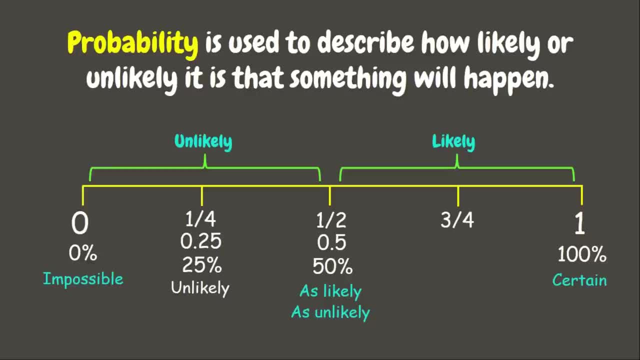 For example, if the probability is 3 fourths, which is 0.75 or 75%, the likelihood of the event to happen is likely, since it's between 1, half and 1, or 50% and 100%. The likelihood of the event to happen is likely, since it's between 1, half and 1, or 50% and 100%. 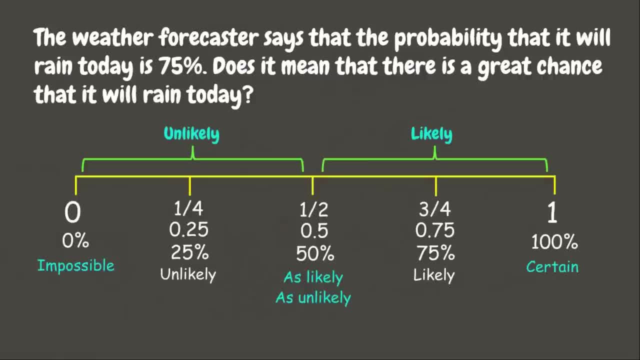 The likelihood of the event to happen is likely, since it's in one-third way than the stays macam. Let's DETERMINE the LISTENING PERCENT of the ELIMINATION of the. It Will Rain Today. Uses probability line to determine the luck it will rain today. 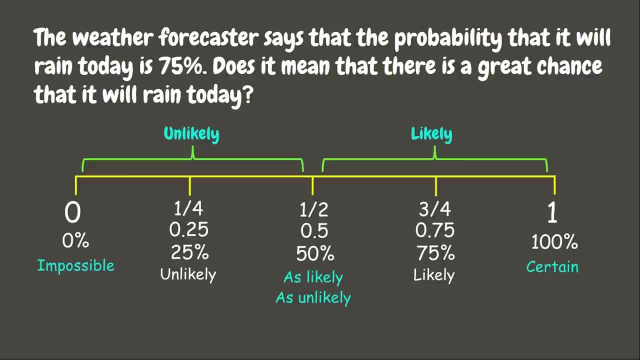 Since the forecaster says 75%, we can say 75% falls between 50% and 100%. This means that the event that it will rain today is likely to happen. Great Job. Now Let's determine the likelihood of the event to happen today. 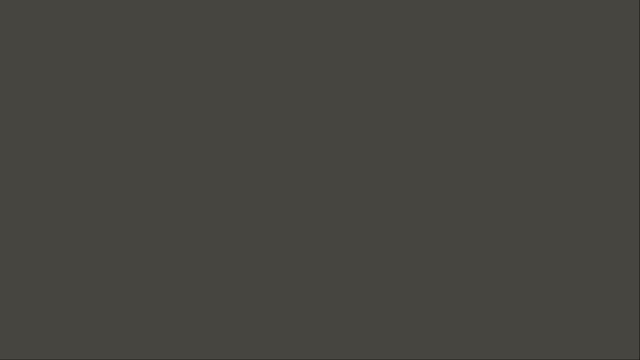 Let's see what probably happens if the 50% falls to 100%. the 55% falls to 1 half. Now Let's Demonstrate and See the risks- ожидentially, likelihood or probability of the following events using our probability line. first is it will snow. 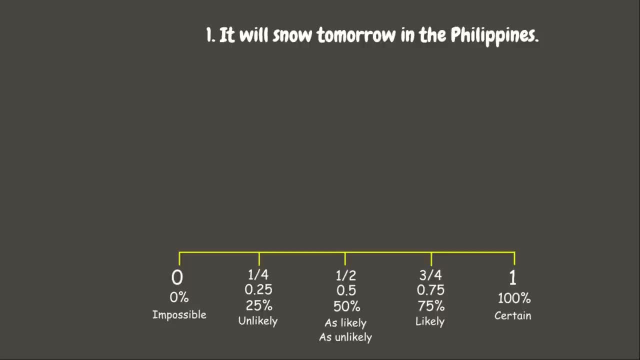 tomorrow in the Philippines. we all know that there's only two seasons in the Philippines, which are dry and rainy season. it means that there's zero probability or it is impossible to snow in the Philippines. second one: the sun will rise tomorrow, since sun rises every day in the morning. 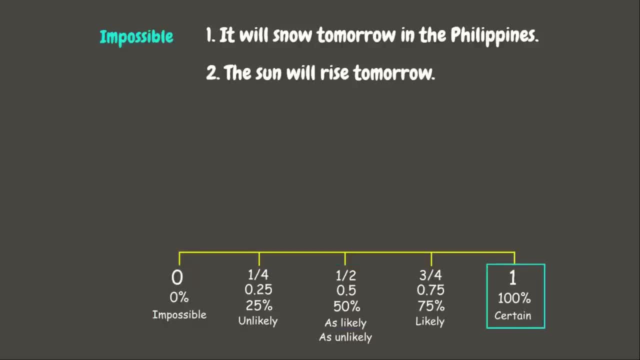 it means that there's 100 probability, or it is certain, that the sun will rise tomorrow. next one: the likelihood that two people in every group of 15 will have the same birthday is eight percent, since eight percent is close to zero and it falls between zero and twenty-five percent. 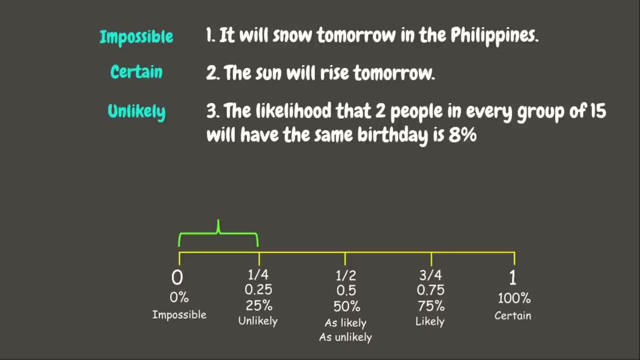 therefore, the event is unlikely to happen. last one sport analyst says that Manny Pacquiao has 85 percent chance of winning. since 85 percent is close to 100 percent, which falls between zero and 75 percent, it means that the event is likely to happen. wonderful. now let's have another example. 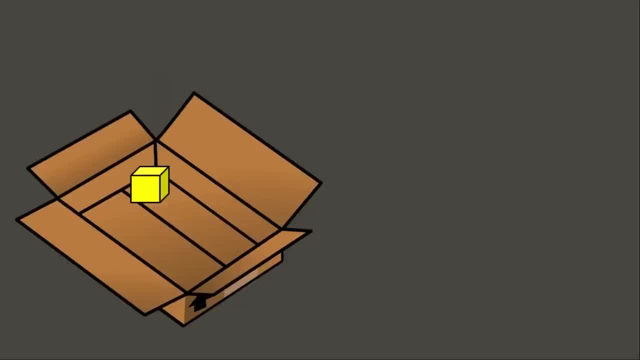 let's say in a box there's one yellow cube, two blue cubes and two green cubes- a total of five cubes. without looking, what is the probability of picking yellow cube out of the book? but how do we get the probability? to determine the probability, we need to divide the number of favorable outcomes by the number of possible outcomes. favorable. 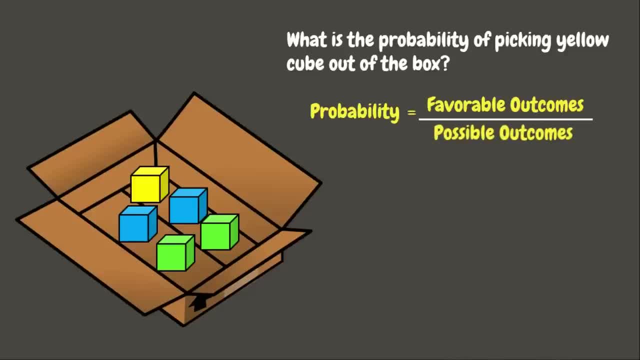 outcomes are the specific outcome you are looking for in the question. we are looking for the probability of picking yellow cube. here we can see that we only have one yellow cube. so that is our favorable outcome divided by the number of possible outcome, which is the total number of all the possible. 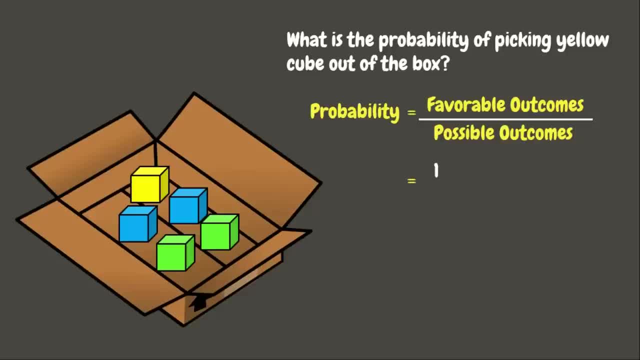 outcomes in an event. Here we have the sample space, or the least of the total number of all the possible outcomes, which are 1 yellow, 2 blue and 2 green, a total of 5 cubes. It means that we have 5 possible outcomes. Now, in a fraction form, the probability is 1. fifths. 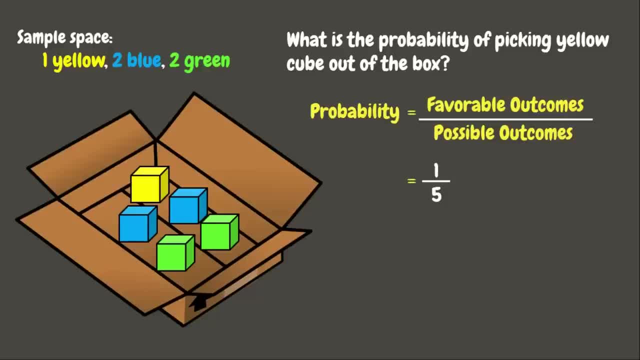 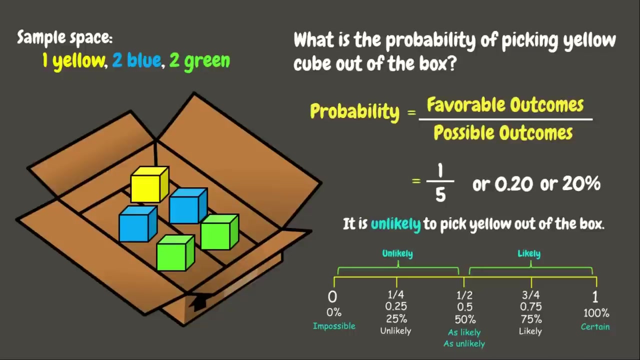 To convert this to decimal, just divide 1 by 5, which is 0.20 or 20 percent In the probability line. the likelihood of this event is unlikely to happen, since it is closer to 0 or between 0 percent and 50 percent. Wonderful, Let's have another question Now. what if we are? 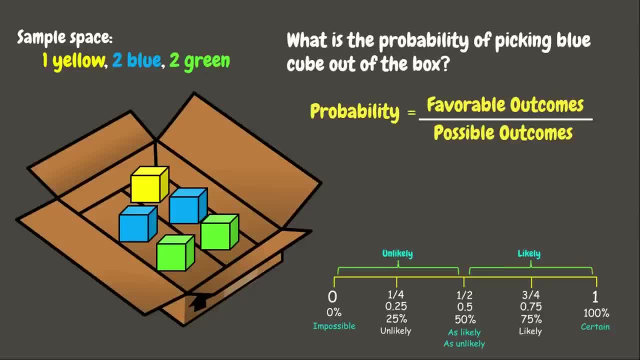 looking for the probability of picking blue cube. I'll tell you how to do it. First, we need to find the probability of picking blue cube. Now, what if we are looking for the probability of picking blue cube? I'll tell you how to. do it. First we need to find the probability of picking blue cube. Here in this now bar we will write 1 plus the proper number of possible outcomes. Here 1 plus 2 is equal to 0.22 and 0.28.. 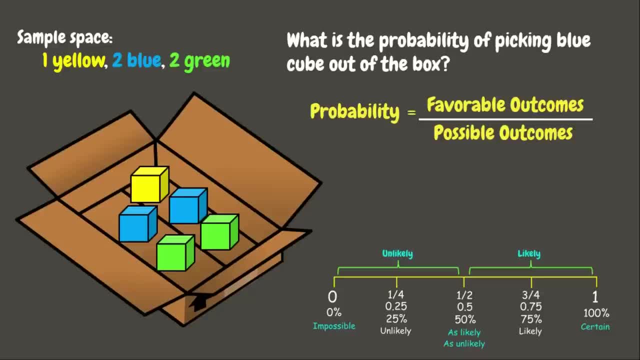 First divide the probability by Mateoous. Let's say the total number of possible outcomes has to be 0.02, which this minutes. So now we add next to 0.2, 0, until we have the possible equals dream. Now it means to divide 1 square. Let's start with 1000.. 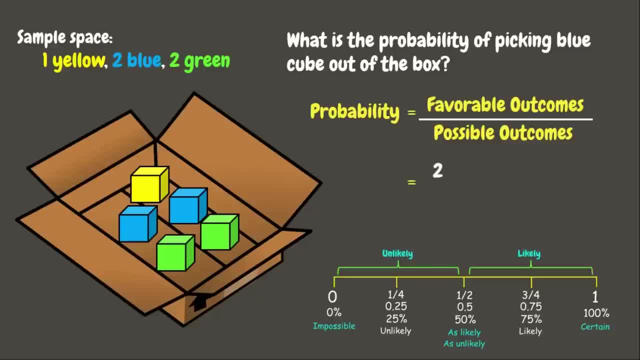 In this picture. it will be the probability of picking the blue cube. So now let's divide thisício 70 by 50 and this 20 y in the other box. Now in a fraction form, the probability of this is 1 fifths. Here we have 1 fraction. 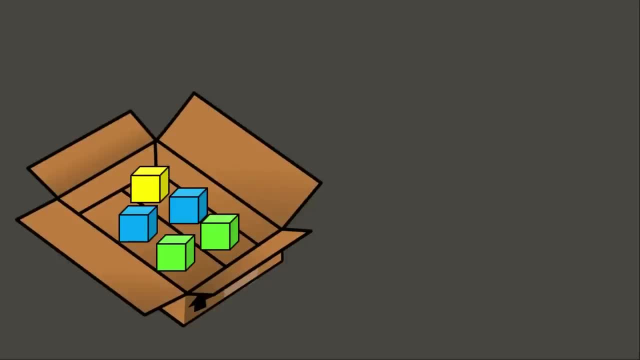 two blue cubes and two green cubes, a total of five cubes. without looking, what is the probability of picking yellow cube out of the box? but how do we get the probability? to determine the probability, we need to divide the number of favorable outcomes by the number of possible outcomes. 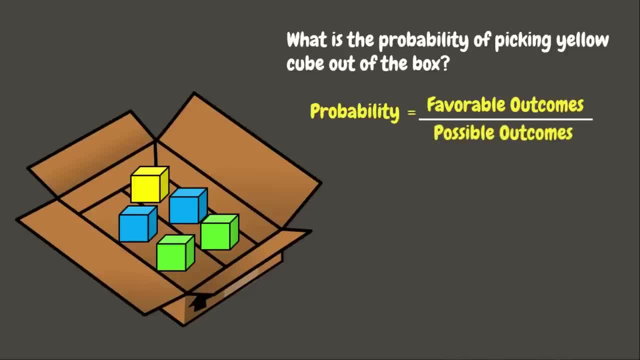 favorable outcomes are the specific outcome you are looking for in the question. we are looking for the probability of picking yellow cube. here we can see that we only have one yellow cube. so that is our favorable outcome divided by the number of possible outcome, which is the total number of all the possible outcomes in an event. here. 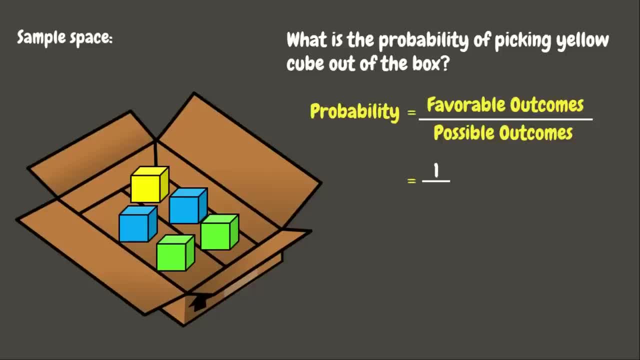 we have the sample space or the least of the total number of all the possible outcomes, which are one yellow, two blue and two green, a total of five cubes. it means that we have five possible outcomes now in a fraction form. the probability is one fifth. to convert this to decimal, 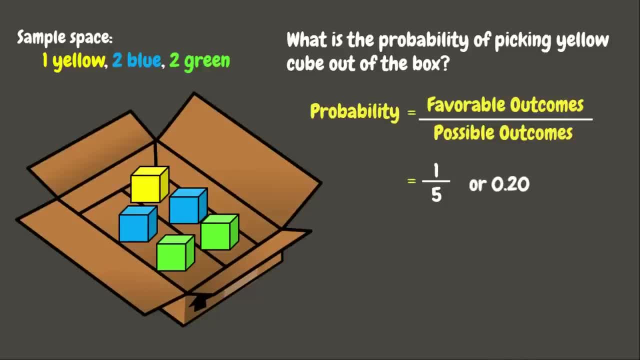 just divide one by five, which is zero point one or twenty percent in the probability line, the likelihood of this event is unlikely to happen, since it is closer to zero or between zero percent and fifty percent. wonderful, let's have another question now. what if we are looking for the probability of picking blue cube out of the box again to determine the 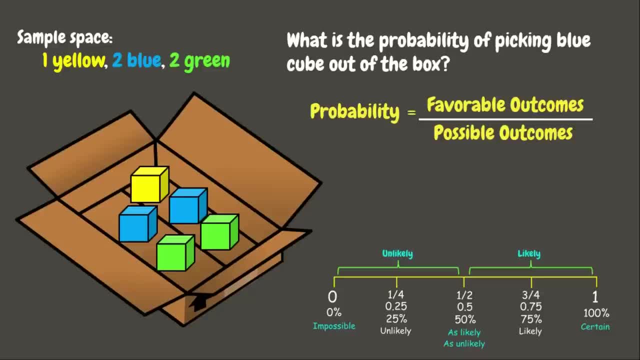 probability, just simply divide favorable outcomes by the possible outcomes. here the favorable outcomes are the blue cube. since we have two blue cubes, it means that we have two favorable outcomes divided by the total number of possible outcomes, which is five. now, in a fraction form, the probability is two-fifths. to convert this to decimal, just divide two by five, which is 0.44. 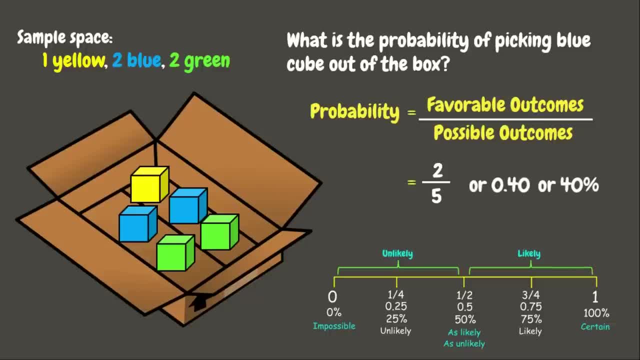 which is 0.4440% In the probability line. the likelihood of this event is unlikely, since it is between 0% and 50%. Next one: What is the probability of not picking yellow cube out of the box? Again to determine the probability? 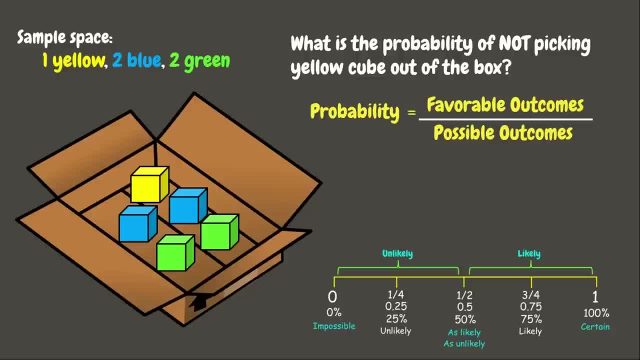 always remember to simply divide favorable outcomes by possible outcome. Here the favorable outcomes are all the cubes except yellow cube. Since we have here 2 blue cubes and 2 green cubes, it means that we have 4 favorable outcomes Divided by the total possible outcomes, which is 5.. 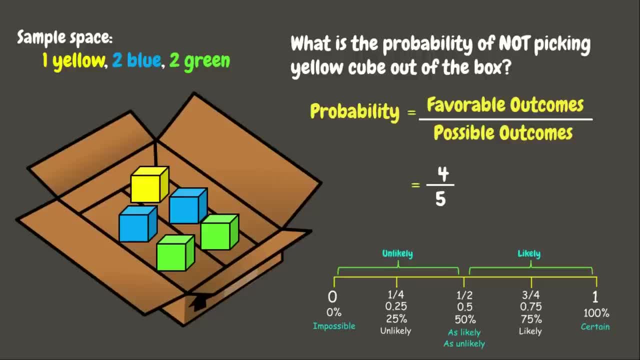 Now in our fraction form, the probability is 4 fifths. Now, to convert this to decimal, just divide 4 by 5, which is 0.8480% In the probability line. we can see that the likelihood of this event. 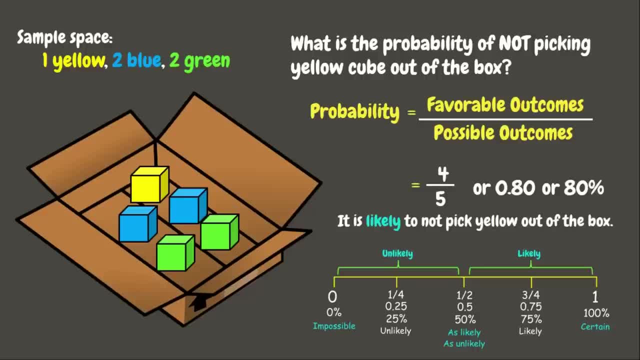 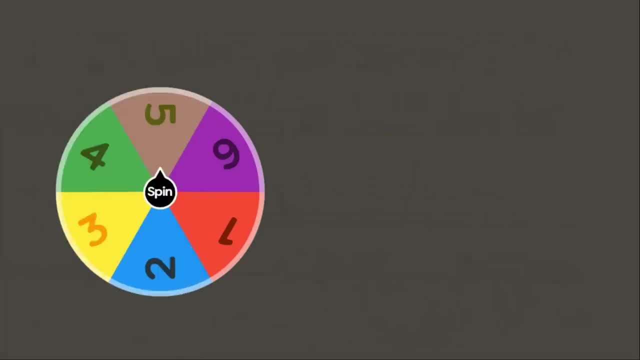 is likely to happen, since it is between 50% and 100%. Wonderful. Let's have another example. This time we have a spinner with numbers 1 to 6. Let's determine the probability of landing on 3 or 5.. 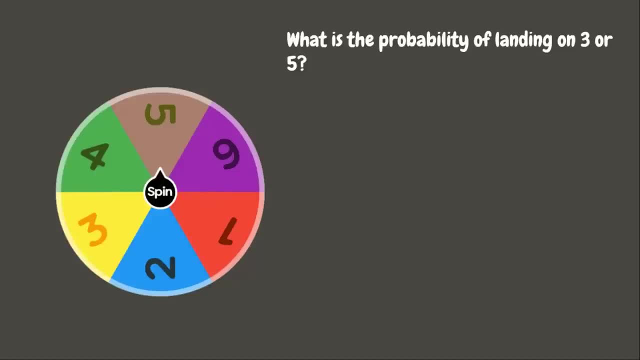 Again, to determine the probability, simply divide favorable outcomes divided by the total possible outcomes. Here we are looking for 3,, 4, 5.. Since we have 1- 3 and 1- 5, it means that we have 2 favorable outcomes. 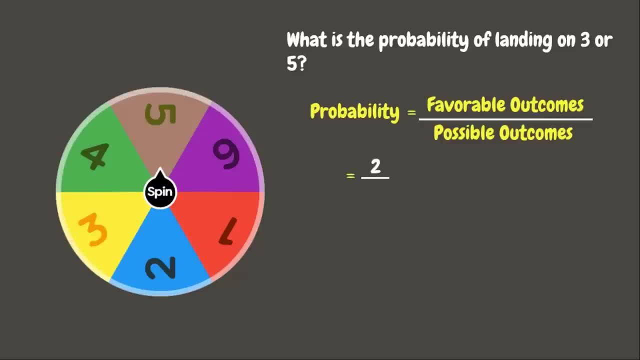 Divided by the total possible outcomes. Here the sample space or the list of possible outcomes are 1,, 2,, 3,, 4,, 5, and 6.. Therefore it means we have 6 possible outcomes Now in our fraction form. 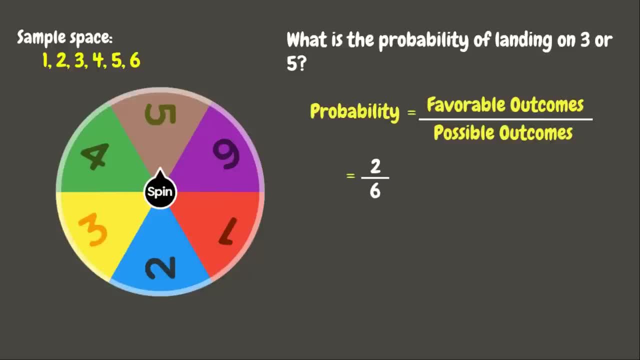 the probability is 2, 6.. Remember, like fractions, we need to simplify this in lowest term. Let's divide this by its greatest common factor, which is 2.. 2 divided by 2 is 1, and 6 divided by 2 is 3.. 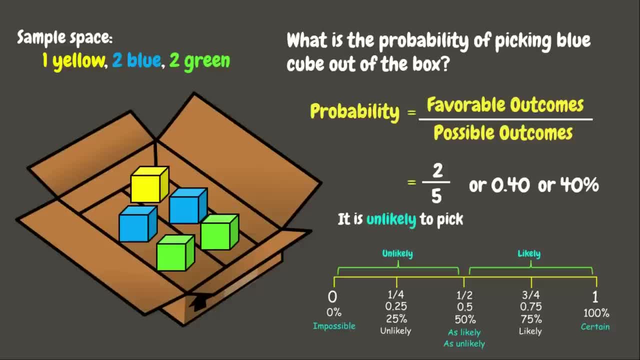 forty percent in the probability line. the likelihood of this event is unlikely, since it is zero percent and fifty percent. next one: what is the probability of not picking yellow cube out of the box again? to determine the probability, always remember to simply divide favorable outcomes by possible outcome. here the favorable outcomes are all the cubes except yellow cube, since we have 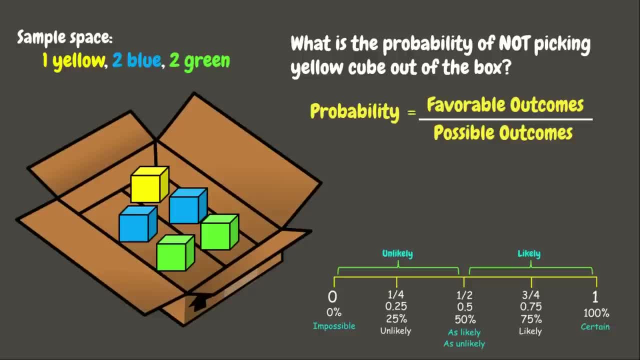 here two blue cubes and two green cubes. it means that we have four favorable outcomes divided by the total possible outcomes, which is five. now, in a fraction form, the probability is four-fifths. now, to convert this to decimal, just divide four by five, which is zero, point eighty. 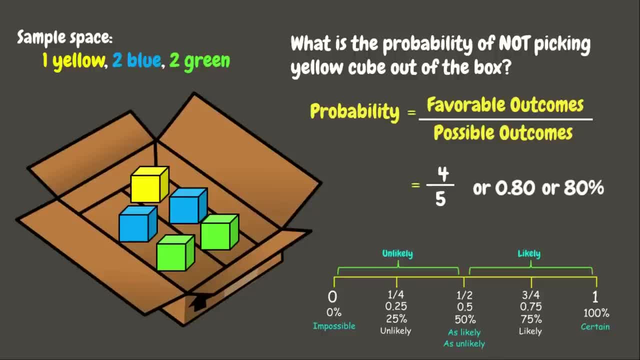 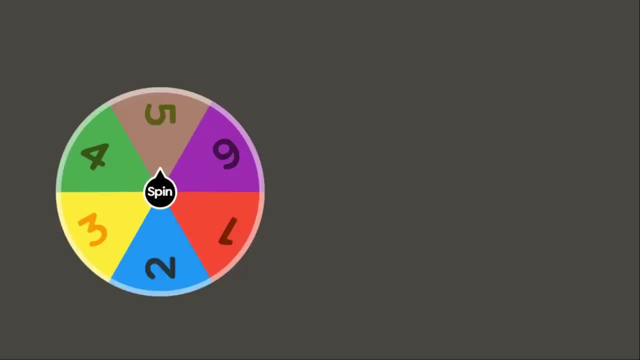 or eighty percent in the probability line, we can see that the likelihood of this event is likely to happen, since it is between fifty percent and one hundred percent. wonderful, let's have another example. this time we have a spinner with numbers one to six. let's determine the probability of landing on three or five. again to determine the probability. 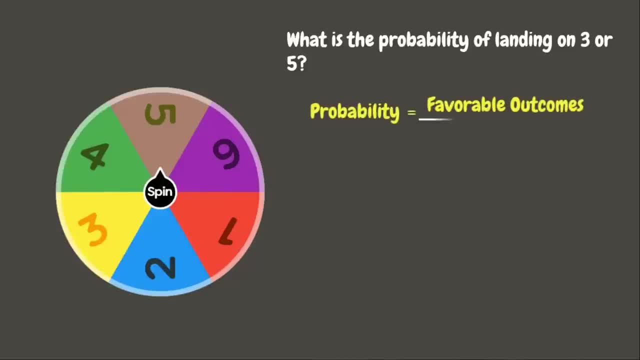 simply divide favorable outcomes by the total possible outcomes. here we are looking for three, four, five. since we have one three and one five, it means that we have two possible outcomes divided by the total possible outcome. here the sample space or the list of possible outcomes are one, two, three, four, five and six. therefore it means we have six possible. 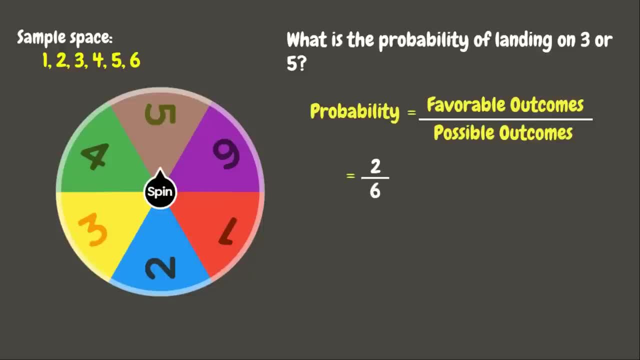 outcomes. now, in our fraction form, the probability is two- six. remember, like fractions, we need to simplify this in lowest term. let's divide this by its greatest common factor, which is two. two by two is one and six divided by two is three. therefore, the probability in fraction form is: 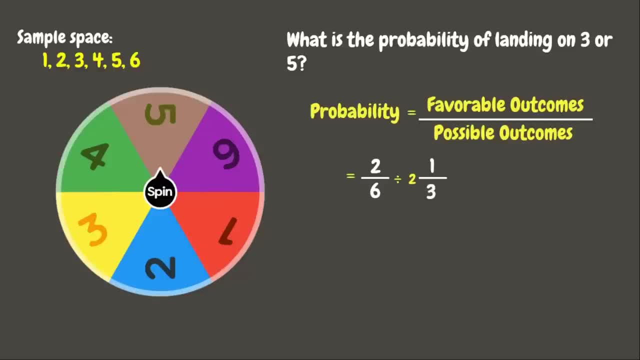 Therefore, the probability in fraction form is 1: 3rd. To convert this to decimal, just divide 1 by 3, which is 0.33 or 33% In the probability line. the likelihood of this event is unlikely, since it is between 0% and 50%. 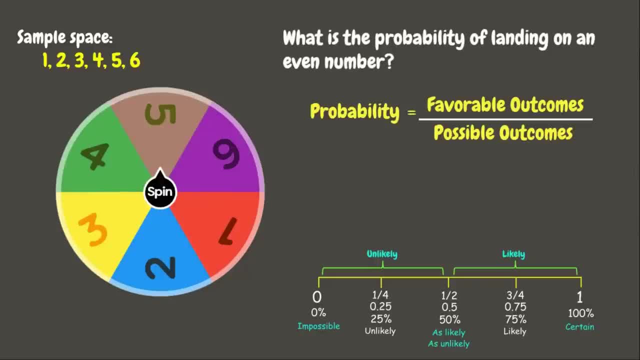 Next one. What if we are looking for the probability of landing on an even number? Here? the favorable outcomes are the even number. The even number on the spinner are 2,, 4, and 6.. Therefore, we have 3 favorable outcomes. 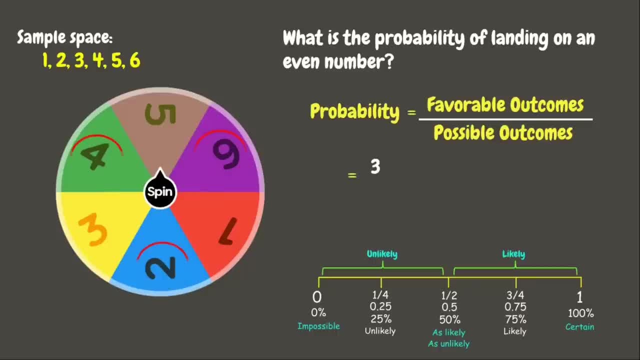 divided by the total possible outcomes, Which is 6.. Again, let us simplify this one by getting its lowest term. We can divide this by its greatest common factor, which is 3.. 3 divided by 3 is 1, and 6 divided by 3 is 2.. 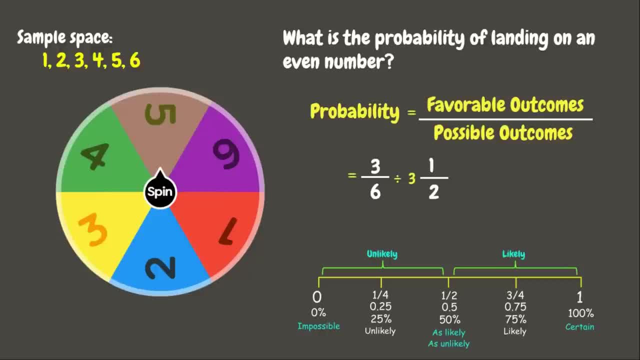 Therefore our final probability in fraction form is 1: 1⁄2.. To convert this into decimal, just divide 1 by 2, which is 0.5454.. Now we can see in our probability line it is either as likely or as unlikely to land on an even number. 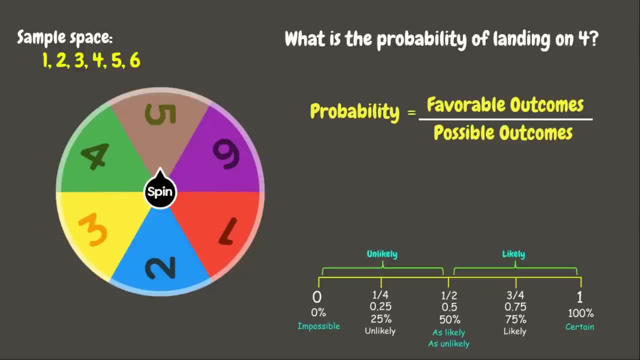 Now let us have another question: What is the probability of landing on 4?? Here the favorable outcome is 4.. And since we only have 1 4 here, it means that we have only 1 favorable outcome divided by the total number of possible outcomes, which is 6.. 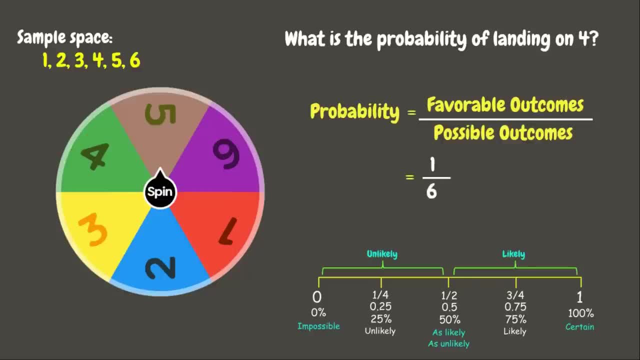 Since we can see that it is already 1, we can see in its simplest form: this is already our fraction form for the probability. Now to convert this to decimal, divide 1 by 6, which is 0.166 or 16.67%. 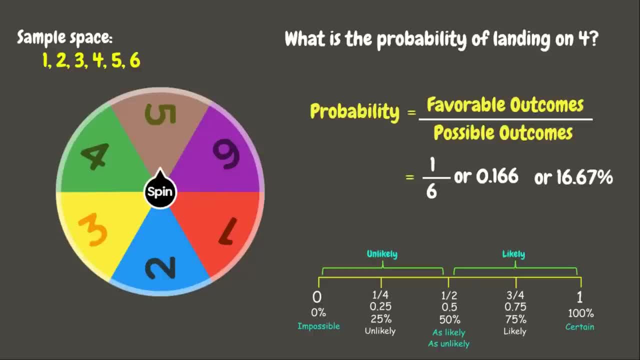 Now again in our probability line, the likelihood of this event to happen is unlikely, since it is between 0% and 15%. Last one: What is the probability of landing on 4?? What is the probability of landing on 4?? 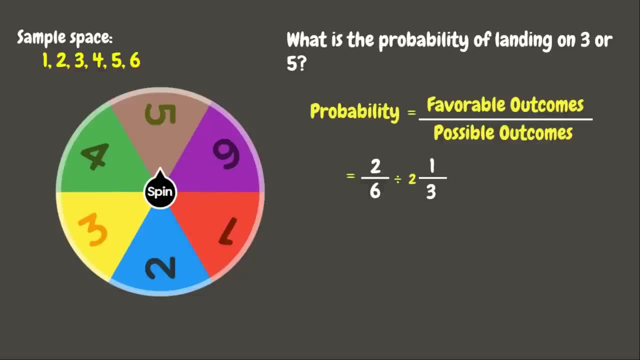 one third. to convert this to decimal, just divide one by three, which is zero, point thirty three or thirty three percent in the probability line, the likelihood of this event is unlikely, since it is between zero percent and fifty percent. next one: what if we are looking for the? 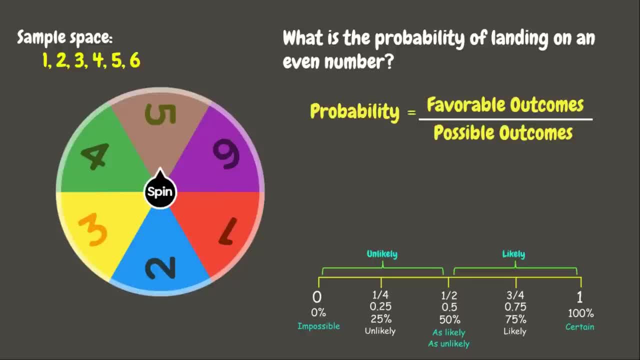 probability of landing on an even number. here the favorable outcomes are the even number. the even number on the spinner are two, four and six. therefore, we have three favorable outcomes divided by the total possible outcomes, which is six. again, let us simplify this one by getting its lowest term. we can divide this by its greatest common factor, which is three. three divided by: 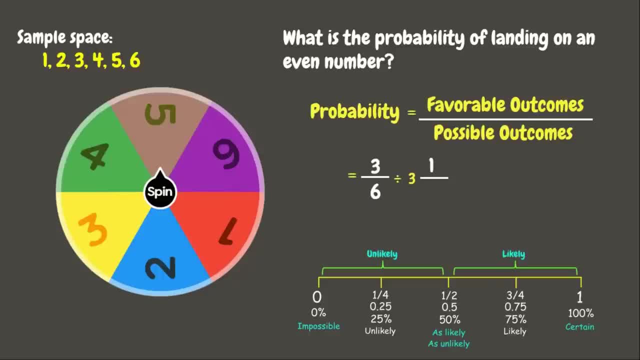 three is one and six divided by three is two. therefore our final probability in fraction form is one half. to convert this into decimal, just divide one by two, which is zero point fifty or fifty percent. now we can see in our probability line. it is either as likely or as unlikely to land. 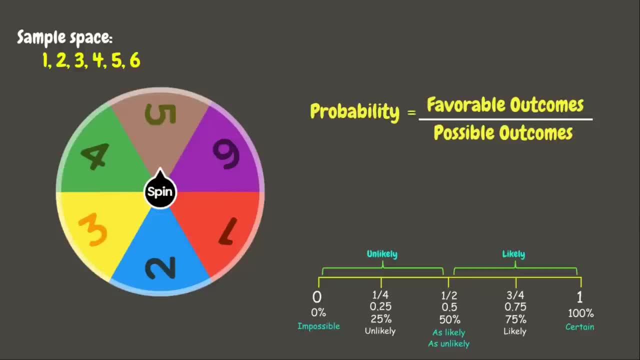 an even number. now let's have another question: what is the probability of landing on an even number here? the favorable outcome is four, and since we only have one four here, it means that we have only one favorable outcome divided by the total number of possible outcome, which is six, since we 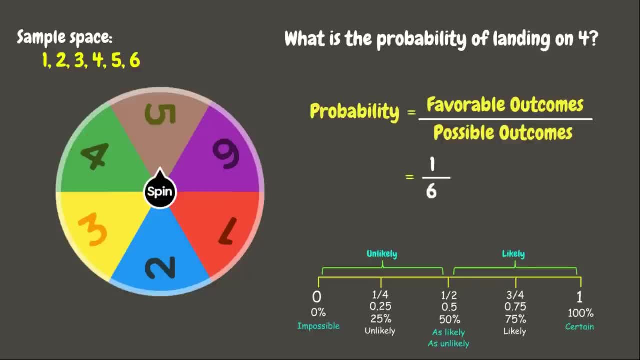 can see that it is already in its simplest form. this is already our fraction form for the probability. now to convert this to decimal divide one by six, which is zero point one, six, six or sixty point sixty seven percent. now, again in our probability line, the likelihood of this event. 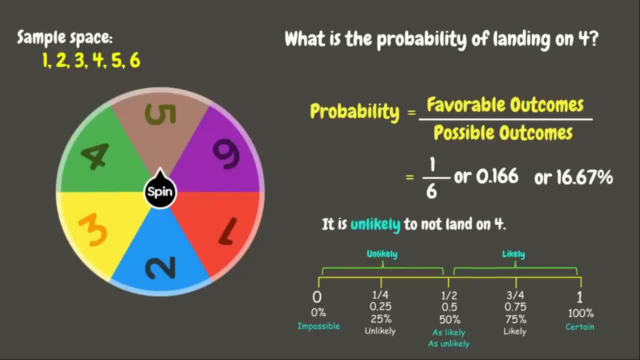 to happen is unlikely, since it is between zero percent and fifteen percent. last one: what is the probability of landing on seven here? the favorable outcome is number seven, but since there's no seven in the wheel, it means that we have zero favorable outcome divided by the possible outcome, which is: